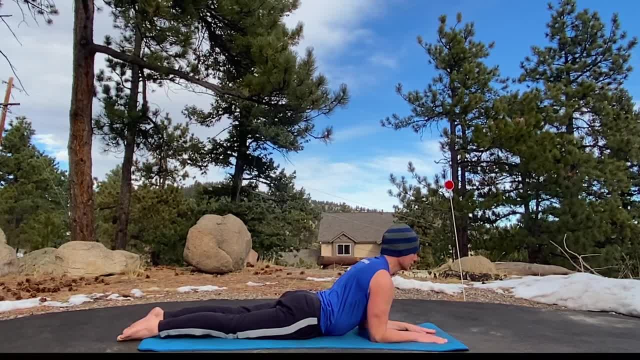 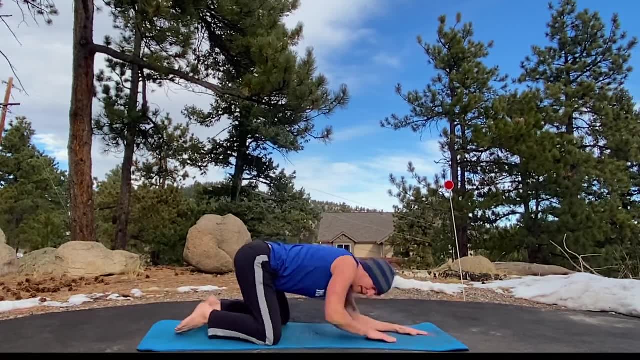 And one more breath. Ah, it's a beautiful thing. I'm going to add something in here. Let's take it back again to the child's pose. Let's thread the needle. This pose is too darn good to just pass up. 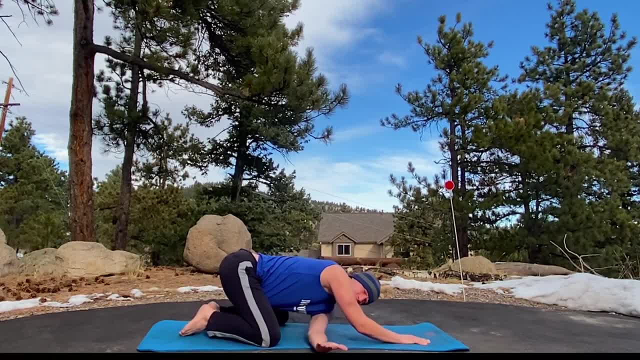 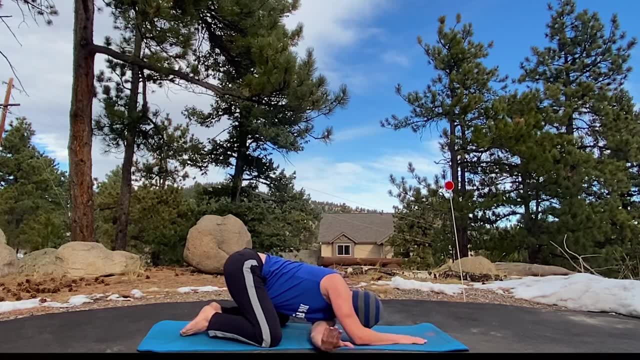 Bring the left arm underneath, This right arm comes forward And now, using your body weight and the gravity, we're going to sink down. So we're stretching the shoulder, the left shoulder, getting a stretch in the spine and a twist. Let's do three breaths right here. 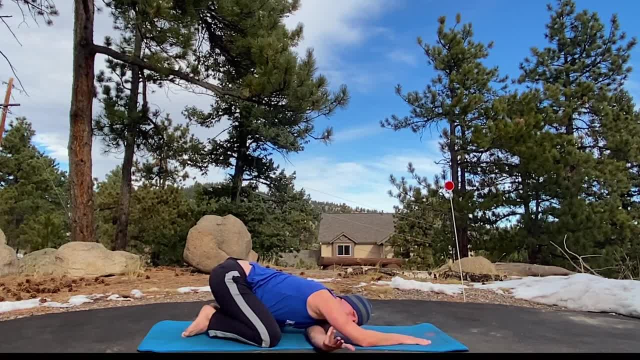 And if you want to see more Yoga for Men videos on this channel, let me know below. I've already done quite a few. I know they're very well received. I love getting more and more guys into the practice of yoga. Okay, walk it up. 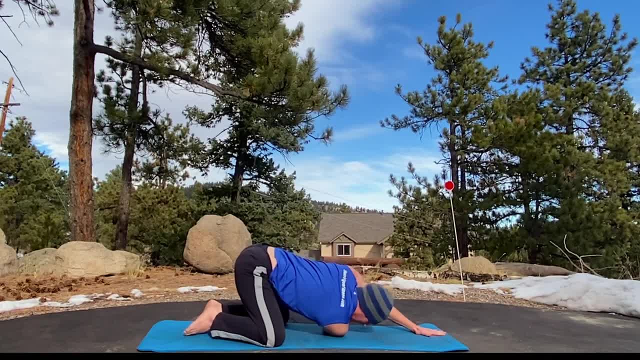 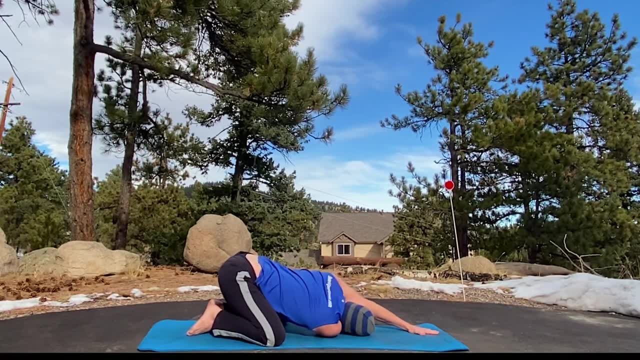 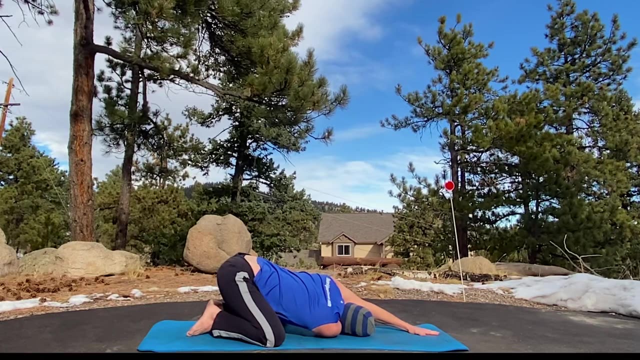 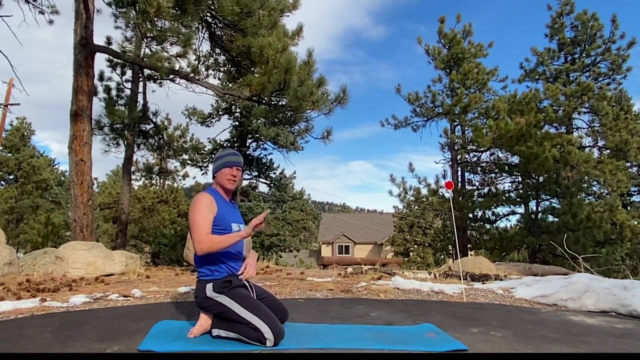 And let's go to the other side: Right arm underneath, Thread the needle, Take three breaths, Good, Deep breathing. We have a nice breeze going, We have the snow, We have the sun. It's a perfect day. All right, the reverse scorpion. 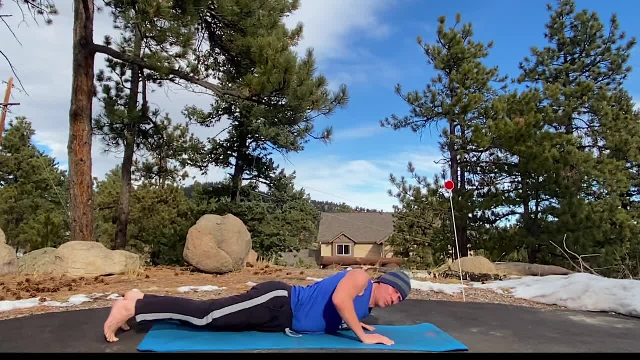 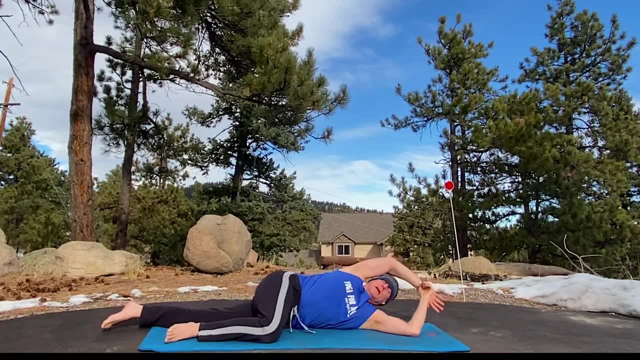 You're going to love this one. This one's going to euthan and open up your low back. You want to take this right arm up and over, pull the cap down and bring the right knee in. So we're coming into a twist. 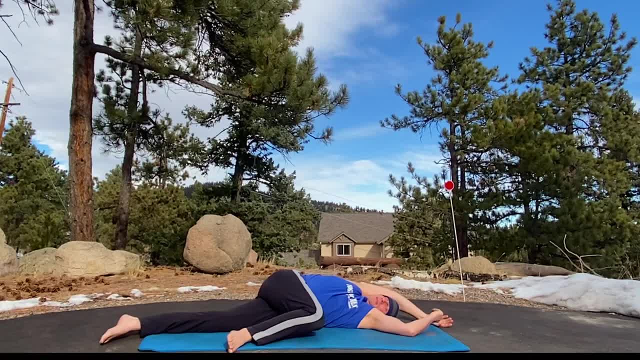 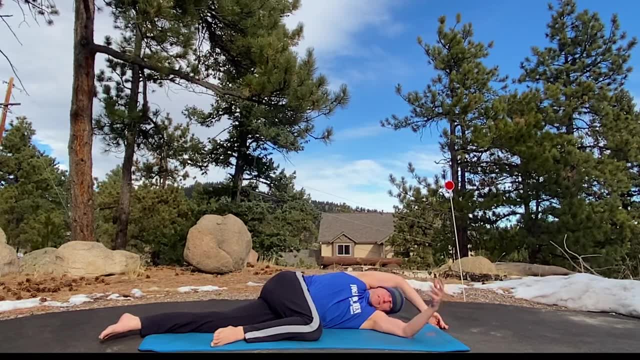 You can also take the arm back here for a little more support, Or extend this leg out In any yoga pose. there's a pose and then there's the extension of it. There's the add-on, if you wish. So right now, relaxing that back shoulder down. 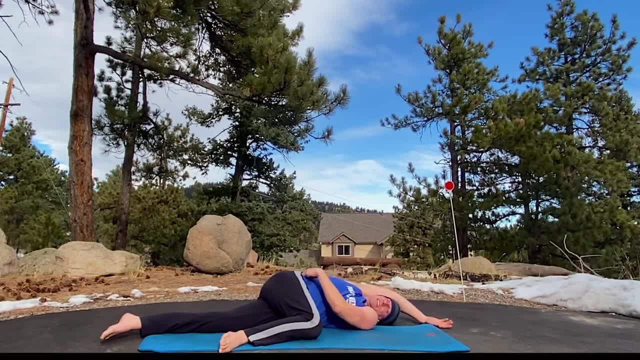 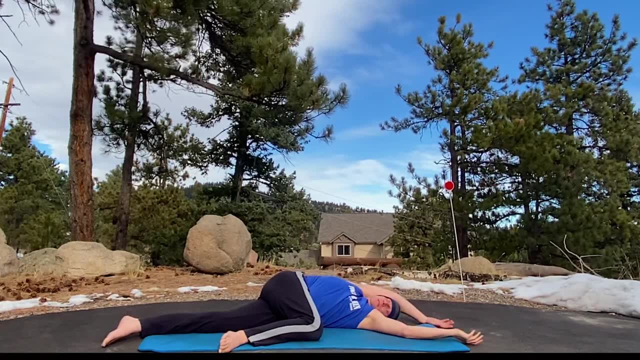 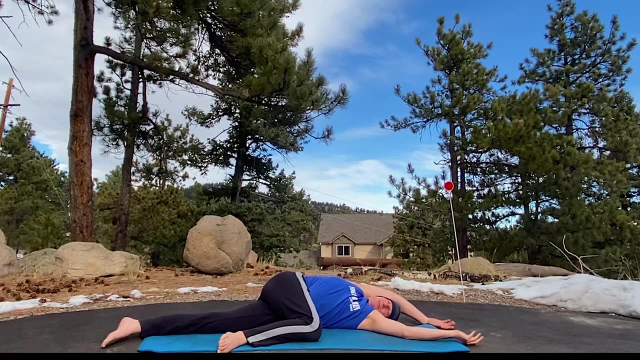 This arm's here for some support. You're getting a fantastic- It's a fantastic, fantastic twist right here. We're opening up the spine and twisting it. Did you get an adjustment? Wind is kicking up. Let's go to the other side. 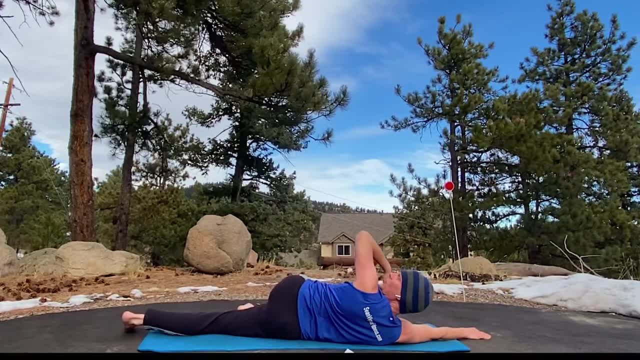 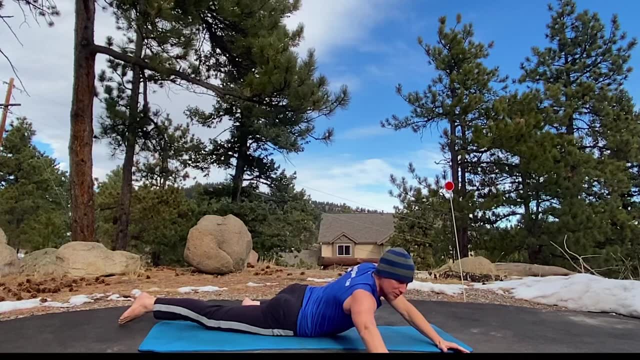 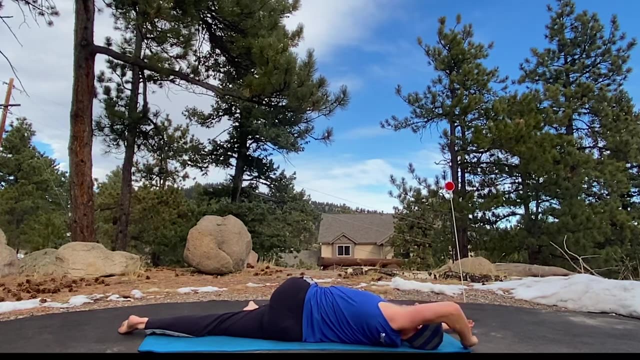 So left arm up and over Left leg forward. Hold that. Uh-oh, there go the notes. You don't want to lose the notes, So worked up, Let's take a few fresh breaths. You want tovised, trimmed x-axis boils and waist. 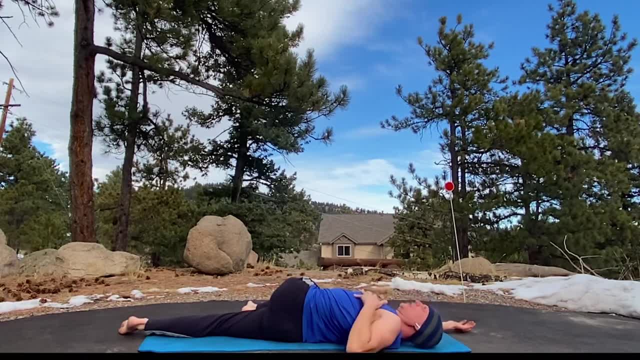 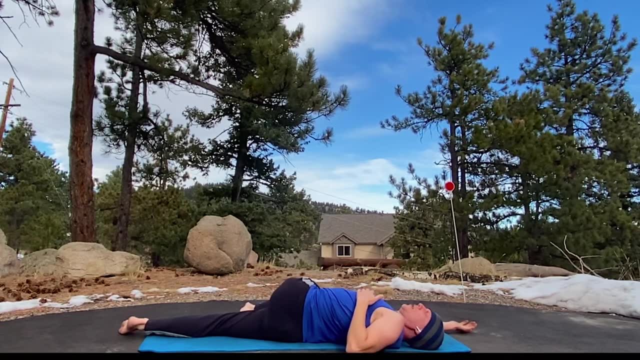 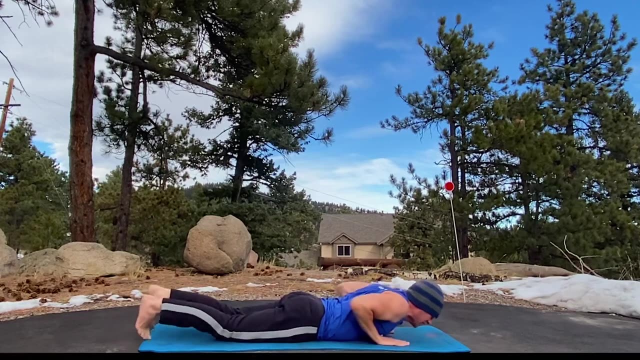 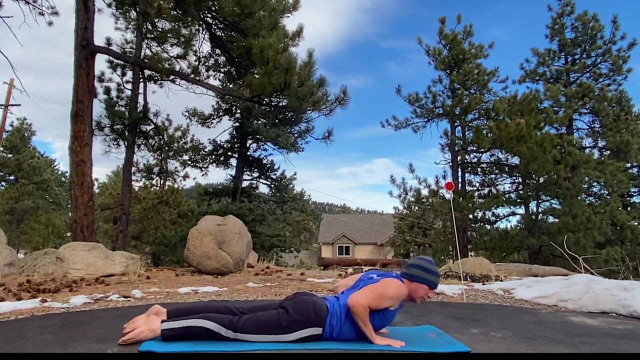 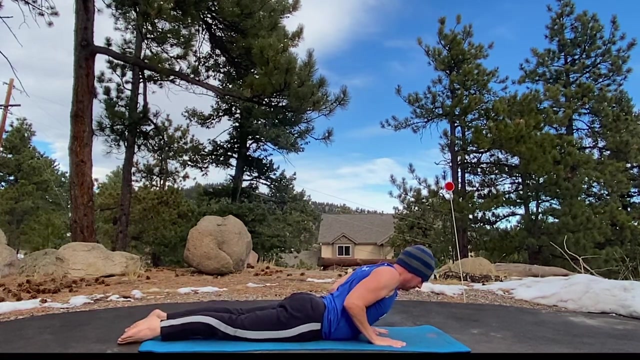 see if that's helping you. There you go, Nice, Hold that for a couple more. Keep down. There we go. Cobra, drawing the shoulders back, lifting into that. Cobra, great for building strength in the back, in the chest, in the abdominals, legs extended- good breathe into it. one. 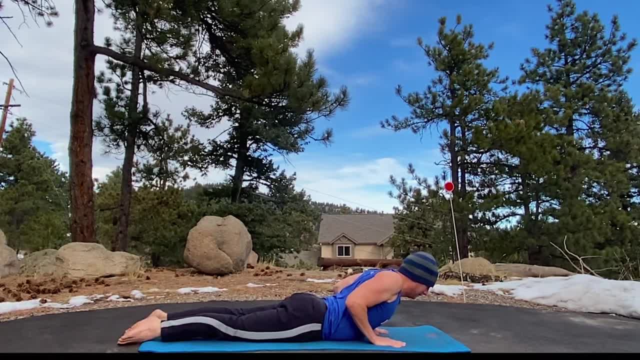 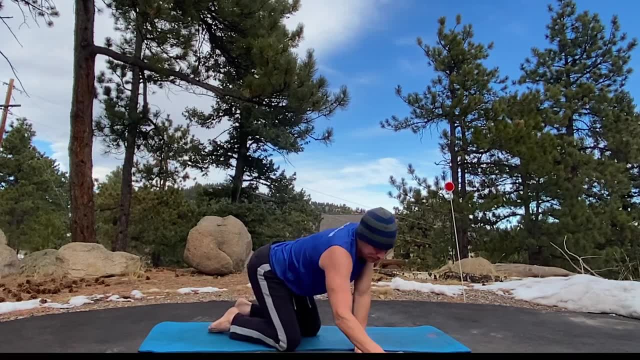 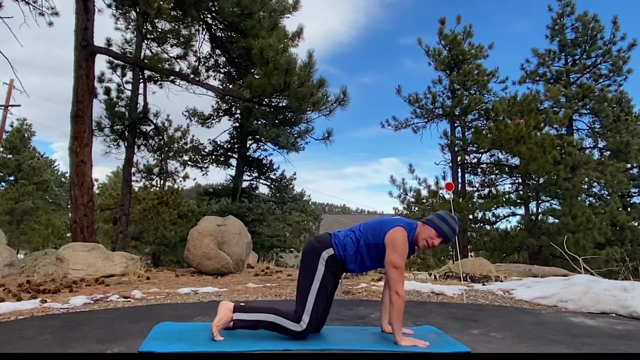 more breath. fantastic, alright, what we're going to do. come to child's pose again, or you can come to a downward facing dog. you're going to take the hands, big, big hands, spread the fingers wide, plant them shoulder width apart. come on up. I want you to bend your. 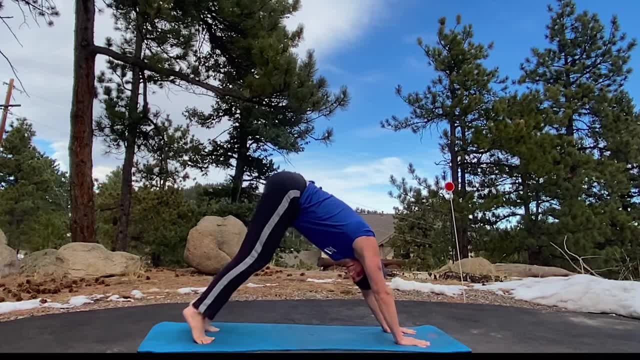 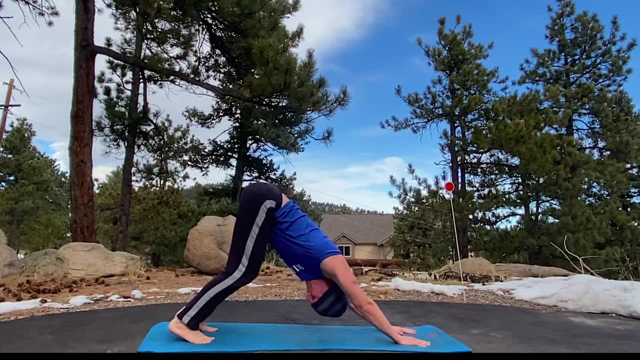 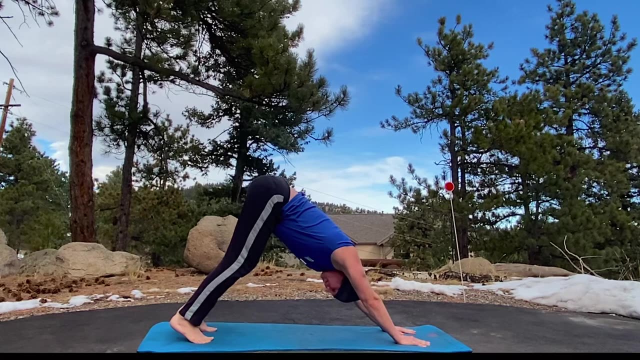 knees here, soften them. so the goal in the down dog is to sink your weight back, to activate the whole back side of your body for a massive stretch. how's that feel? again, you can keep your knees down and work your way up. that's fine, remember, once you get onto the mat. 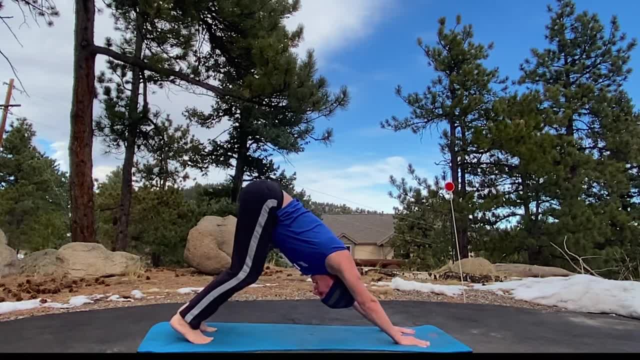 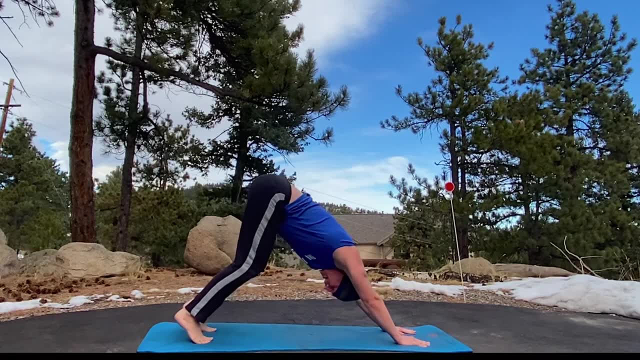 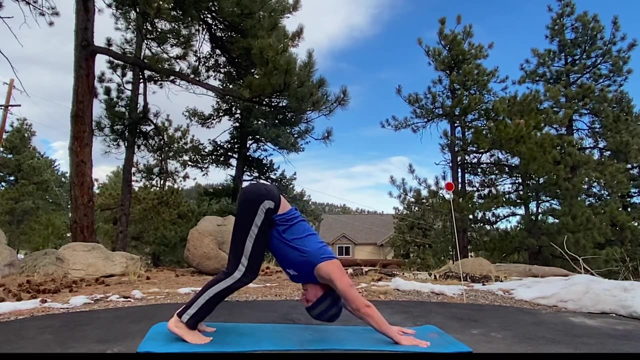 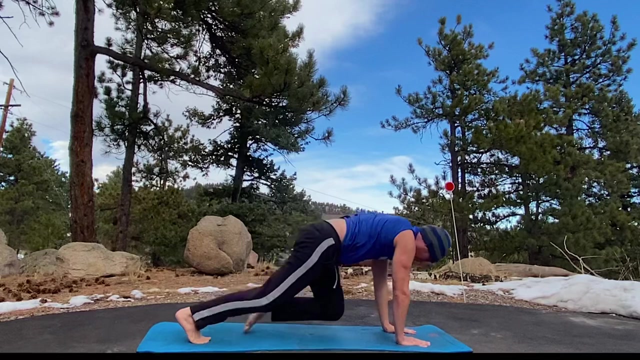 it's your practice, It's all yours, and from here you can lengthen the legs when you're ready. stretching the legs, sinking the heels down, let's do three more breaths. you got a lot of blood coming into the brain, lots of breath to counteract that. okay, bring the knees down, let's come. 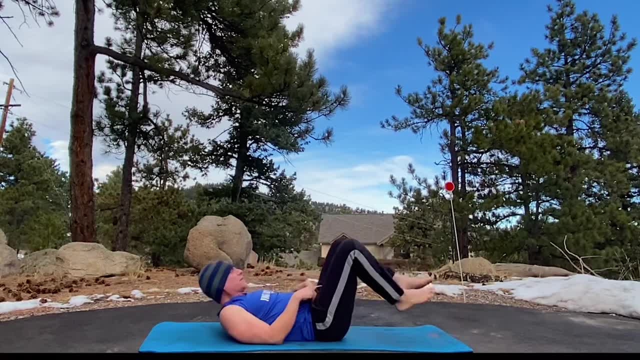 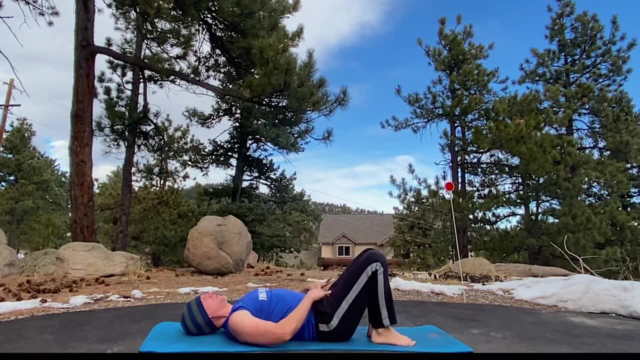 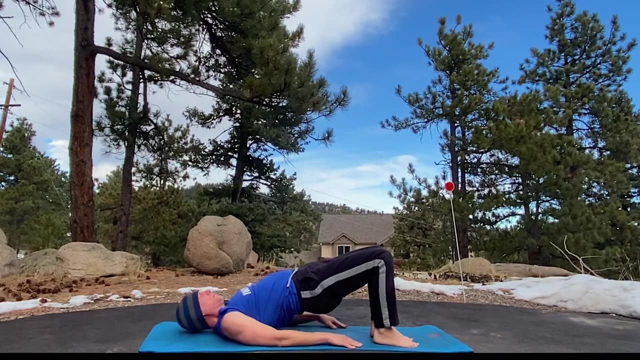 onto our backs, flowing from one pose to the next. We maximize our time, never, ever, wasting a second feet. flat arms to the sides- here's your pelvis, right here. I want you to tilt it up and then lift up into a shoulder bridge. 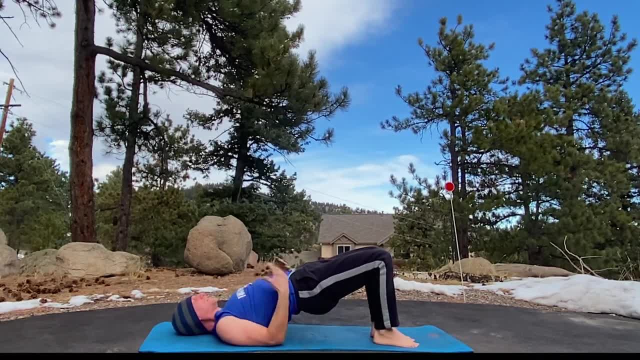 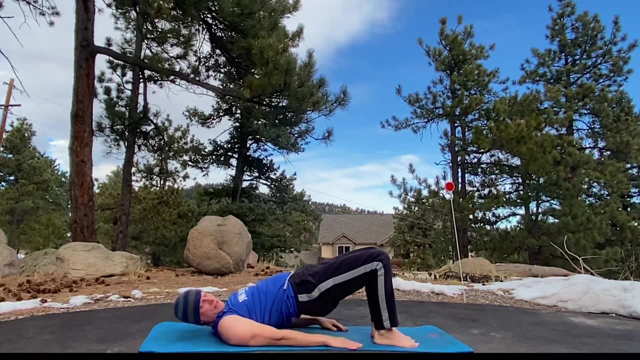 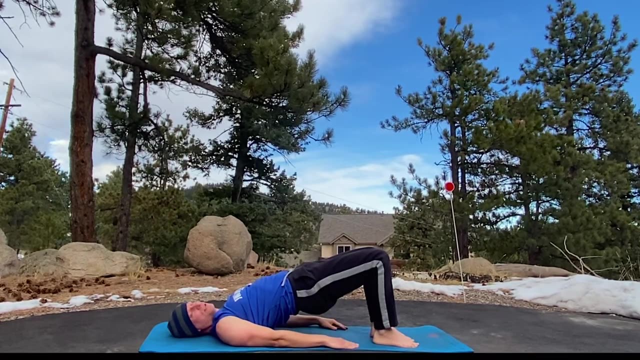 the weight shifts back. we have a nice line here. we're working the glutes and the low back. you could also extend the arms overhead or keep them here. three more breaths. there go the notes. If this is your first time training with me, I usually film outside. I love it, I live. 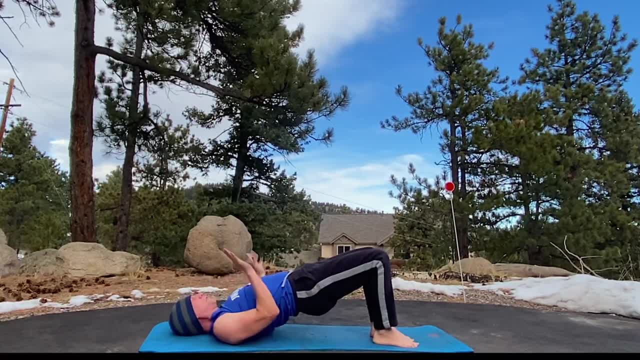 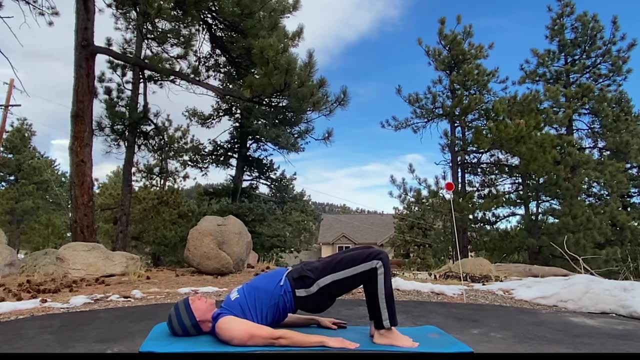 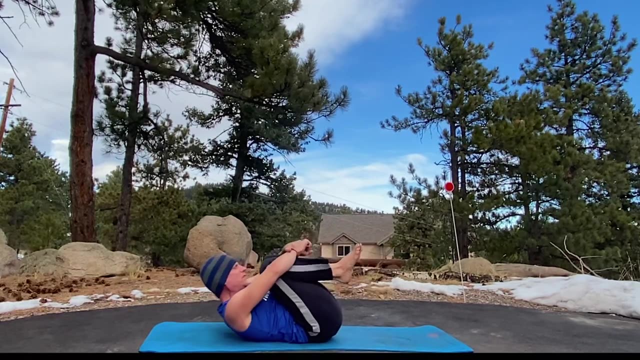 in the Colorado Rockies, so you never know what's going to happen weather-wise, or certain friends coming by- deer elk, you name. it keeps it spontaneous. all right, slowly come down, massage the spine, hug the knees into the chest. oh, this might be your favorite. 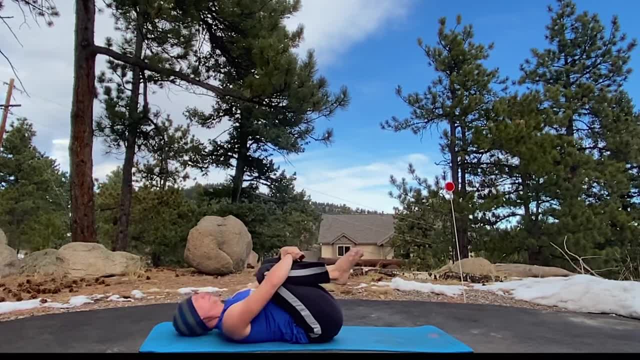 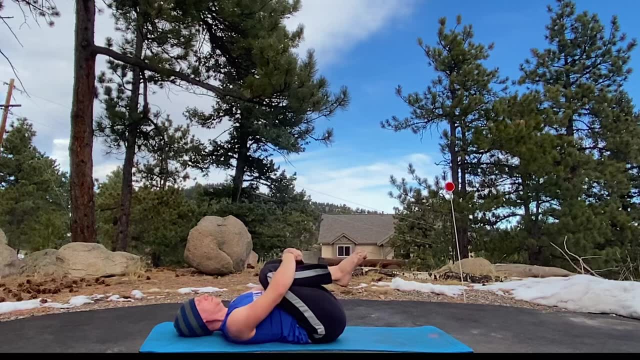 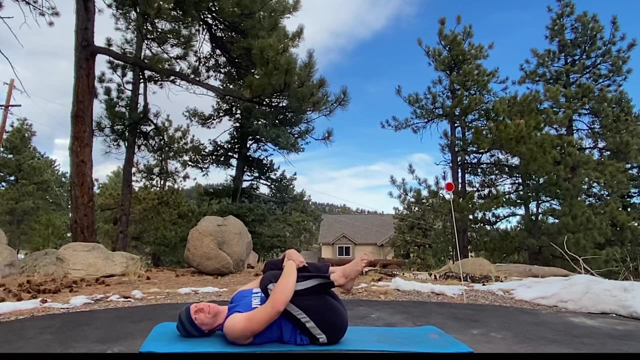 you can always place a pillow underneath your head. five breaths, a little rocking. It's a little rocking side to side, Wiggle the fingers, wiggle the toes again. this is very gentle, this routine, but very powerful. 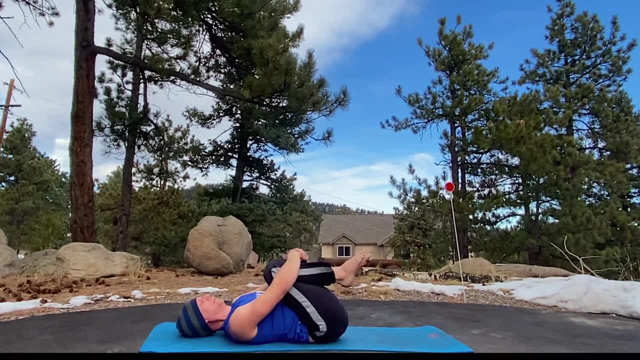 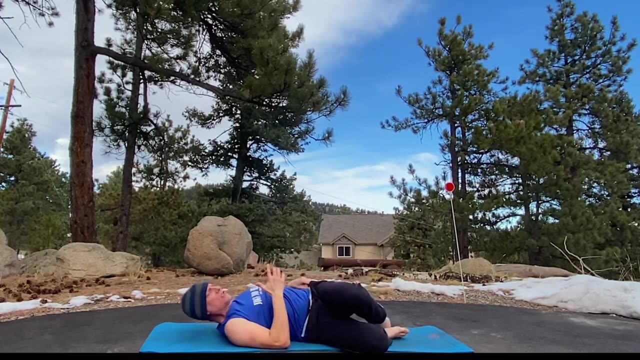 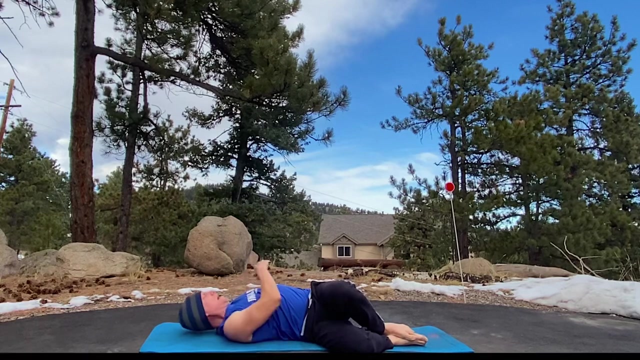 Keep your breath on fire, keep your focus, Keep your moans to yourself. All right, let's drop the legs to the right. the lying spinal twist could extend this top leg out. if you like reaching away, hold for three breaths so you'll find that yoga. 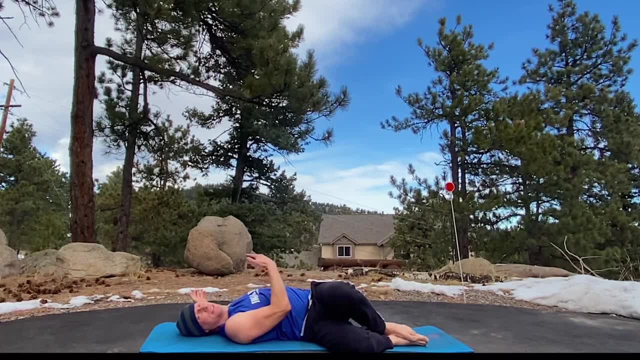 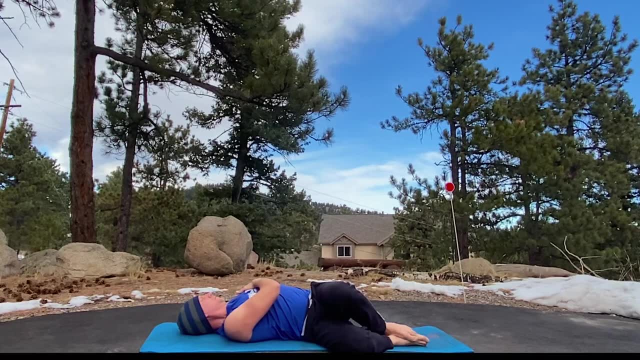 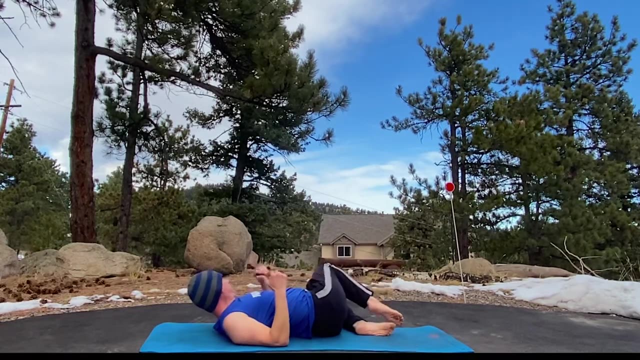 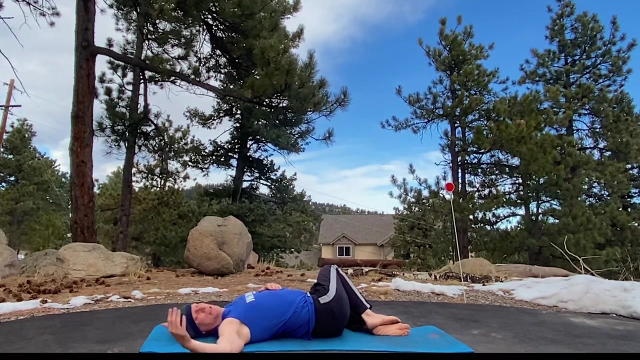 is not some mystery, it's not a conundrum. it's extremely accessible and extremely effective. right here, right now, You feel great and look great immediately. All right other side, look at that big cloud just came in, but nothing shall stop us. 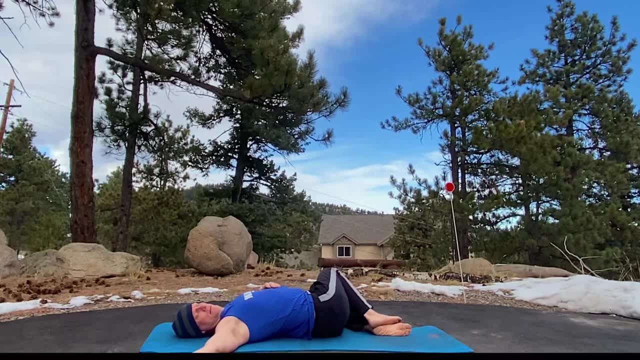 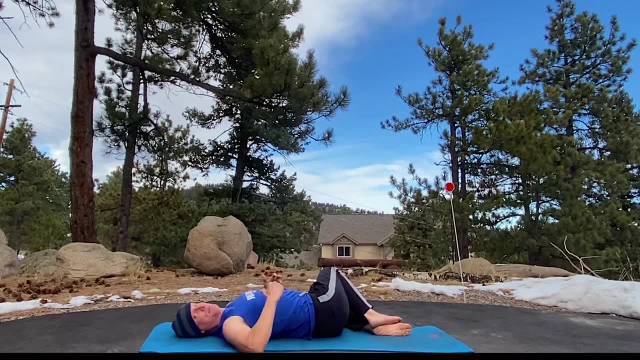 Two more breaths. How is your breath? Keep the breath flowing. you're breathing in and out and to the back. you're always expanding with the breath, No matter what you're doing, from this pose to if you run, if you're sitting and typing. 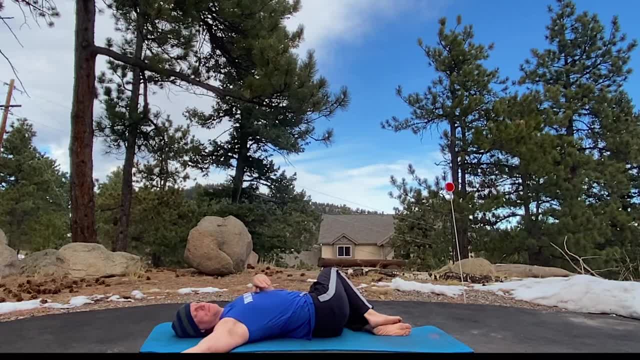 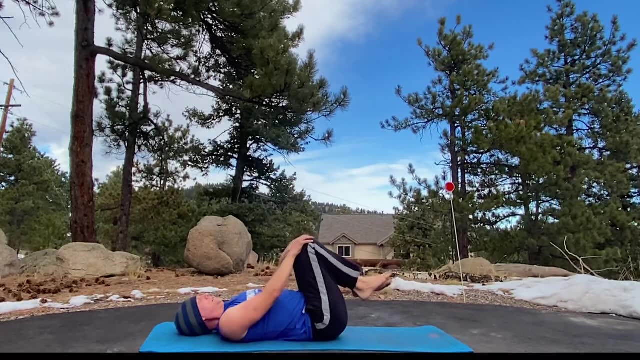 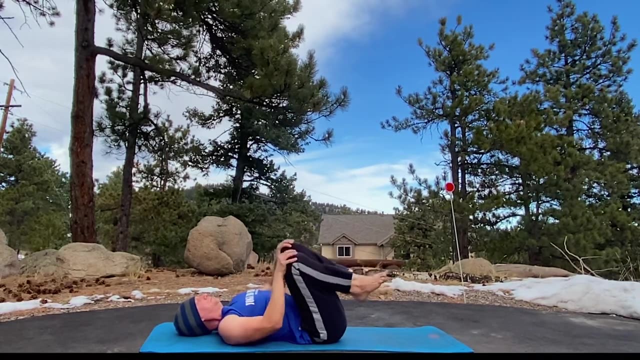 on the computer. you're always breathing. Focus on that breath. All right knees into the chest. Once again, let's circle the knees: one direction, Inhale around, exhale on the top. And other direction: One, two, three. 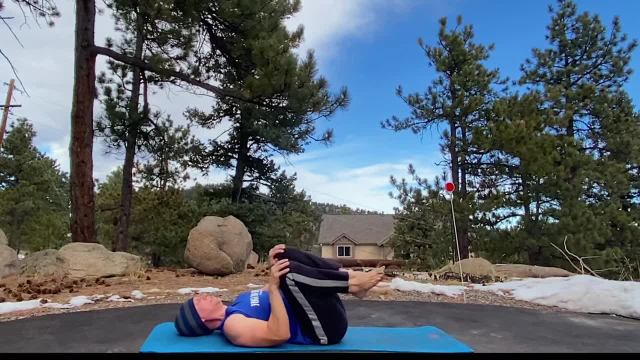 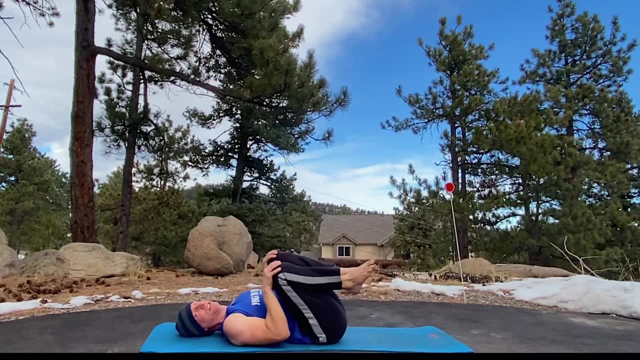 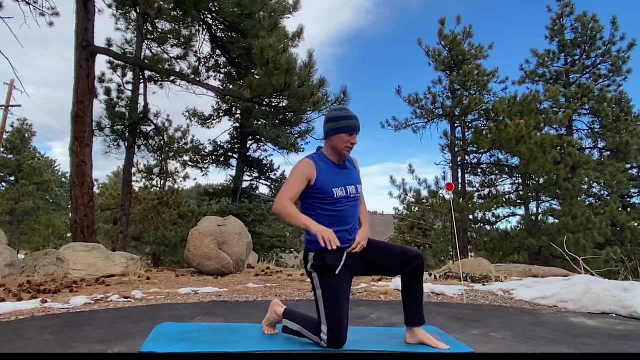 feel good. nice massage for your low back. a lot of times we don't know how bad we need these stretches until we do them. so is life right. so is life all right. let's do one more pose here. my notes have blown about three neighborhoods over, so 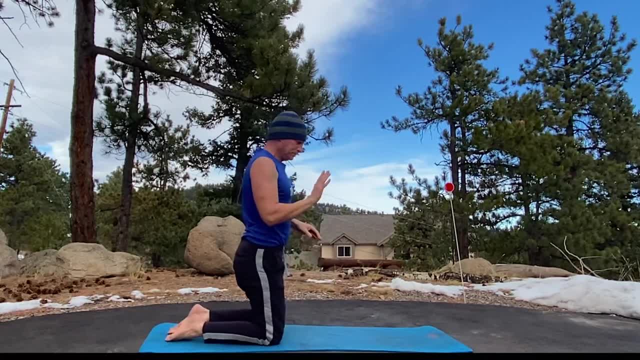 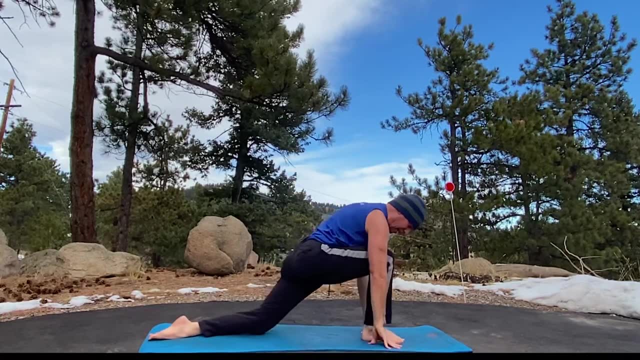 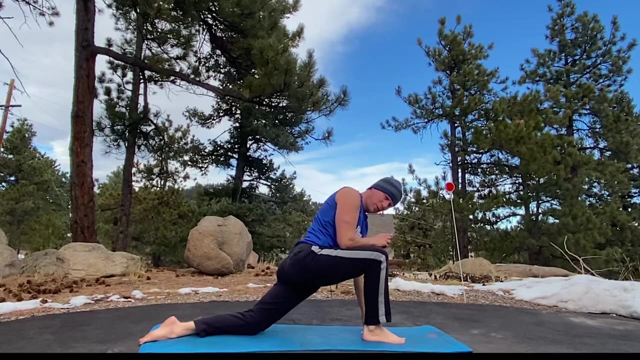 now they're enjoying the beginner yoga: low lunge, low lunge. bring your right foot forward. hands down, this knee can be underneath the hip or slide it back up to you shoulders back. great for activating your front leg, your quad and, very important, you stretch your hip flexor right on the top here, your hip. 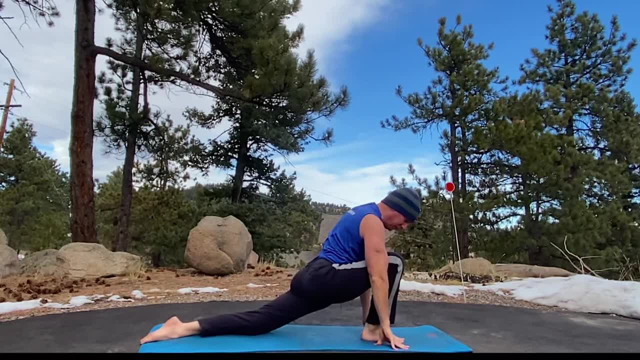 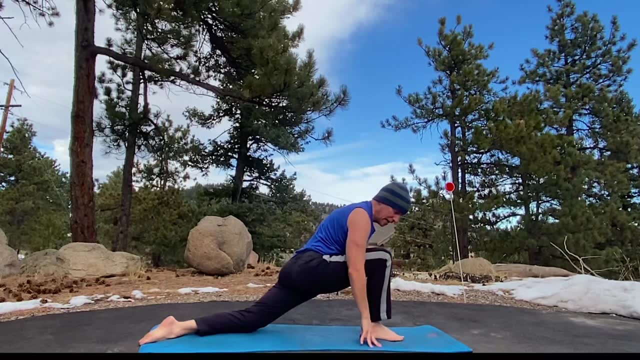 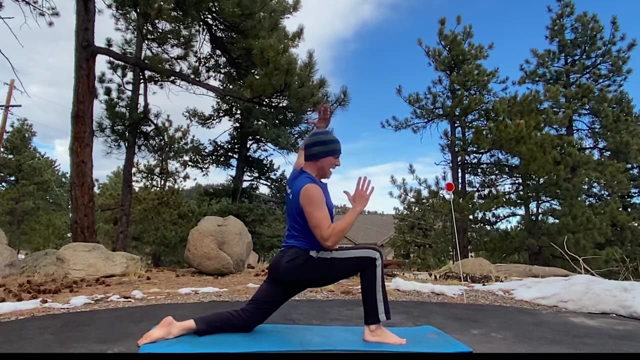 extender on your back leg. feel free to hinge a little bit forward and if you want to add on some more stretch here, we're going to do a little bit of a stretch on the side, for the upper arm broke. warm lying back down and adjusting your armotch themselves. reach up behind teeth on the ground and work your. 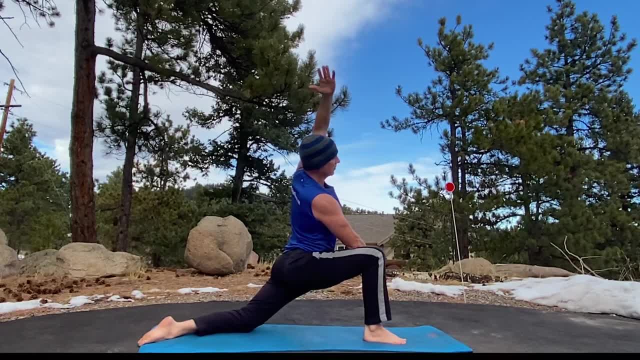 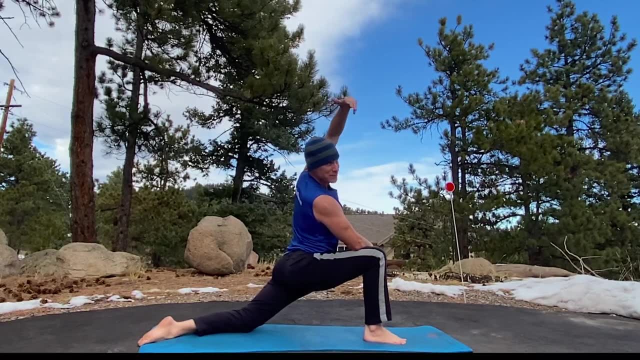 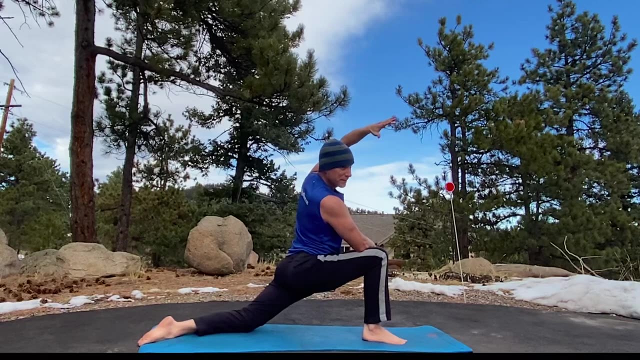 arto this: there's a side bend, bring this forearm here and then this arm comes up and over, when you're ready, of course. so you're activating the core, you're stretching the side, you're working the legs. three more breaths. I like to slip in these little add-ons because, not doing it, you might think I. 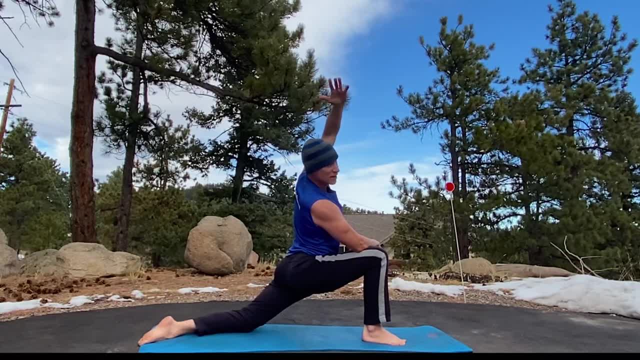 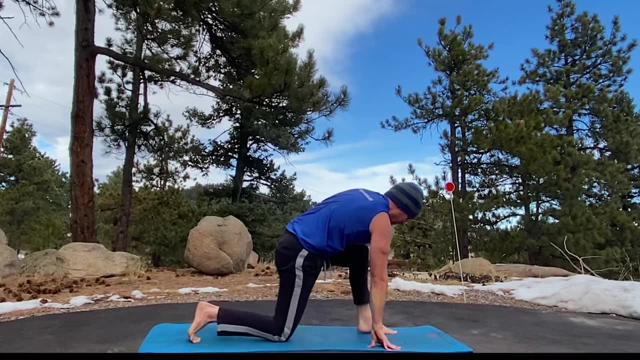 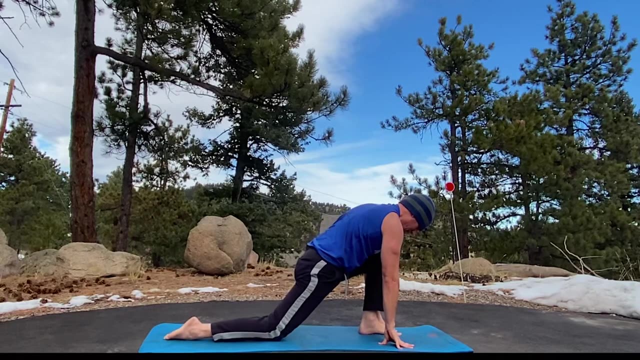 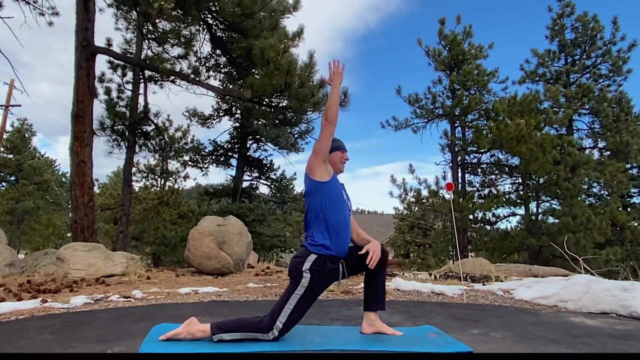 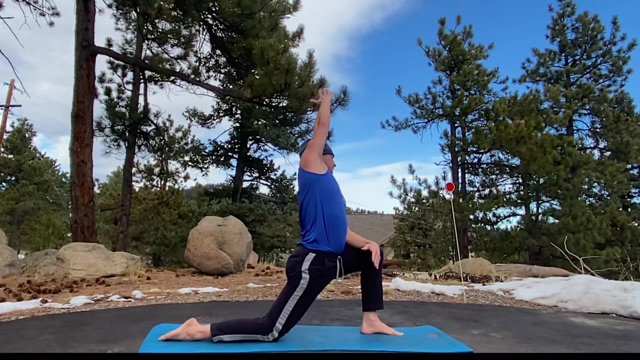 time. it's quite incredible the strides we make in a short amount of time. all right, low lunge, other side doing great, here we are, we're here. if you like, add that side bend, tuck in the shirt. four breaths for good, a living breathing flow.